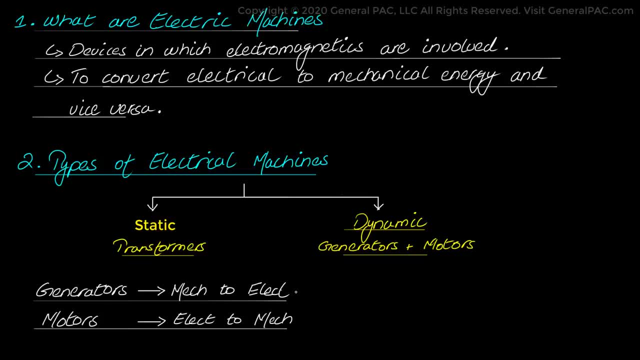 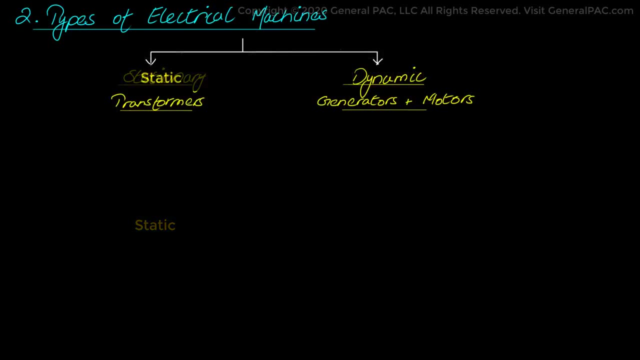 to mechanical energy. This is the basic principles and we all know this. In this series we will focus on generators and motors, because we have already covered transformers in quite a bit of detail. Now, what are the categories of electrical machines? We look at further classification of electrical machines. It is quite conceivable to categorize. 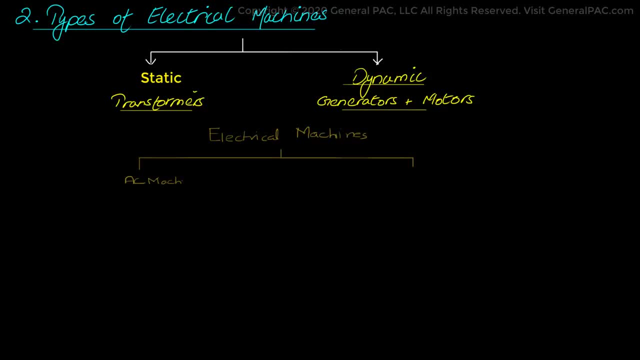 electrical machines based on AC and DC. Here the AC-Machines can be divided into two main types. There is the synchronous machines and the asynchronous machines. In synchronous AC Machinesproducts are composed of two main categories: dystrender and collector. In synchronous AC Machines there are synchronous AC Machines or澤HCоминаqeres, or" pontos. 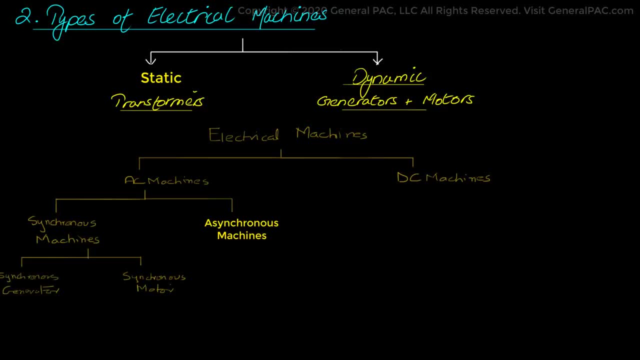 there are synchronous neutrals, orucker machines, alternate, alternates or linear generators and synchronous motors. Then the asynchronous AC machines include induction machines which can be used as an induction motor and induction generator. Similarly, as we can see, there are two types of DC machines. There's the 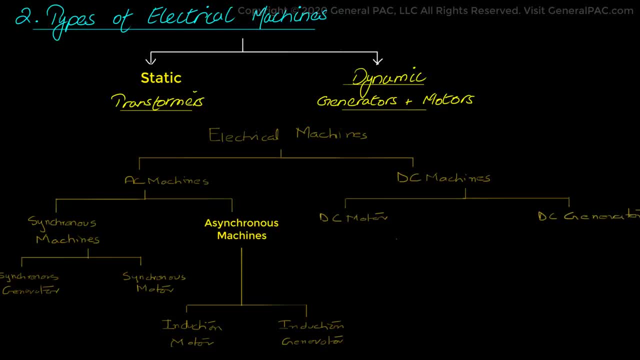 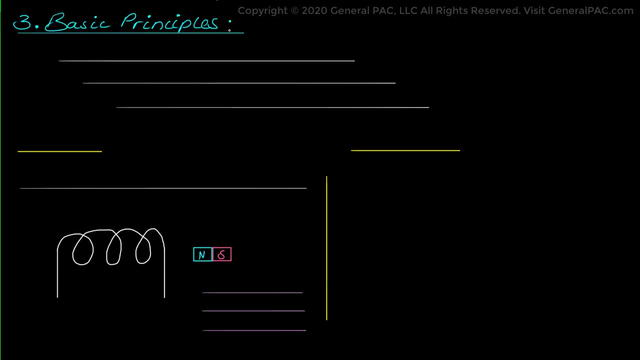 DC motors, and then there's the DC generators. In the end, they can all be used according to either single phase and three phase configurations. Now let's see what are the basic principles involved in electrical machine operation, As we have discussed that machines convert electrical energy to. 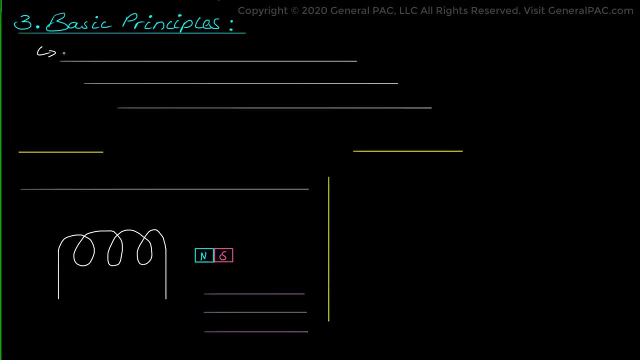 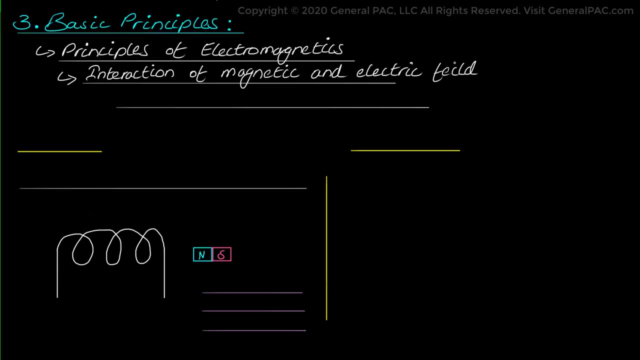 mechanical energy and vice versa, the principles of electromagnetism are applied. In fact, it is an interaction of magnetic fields and electric field and its surroundings which leads to the conversion of energy from electrical to mechanical and vice versa, And this effect is called electromagnetic induction. Now we will have a look at the 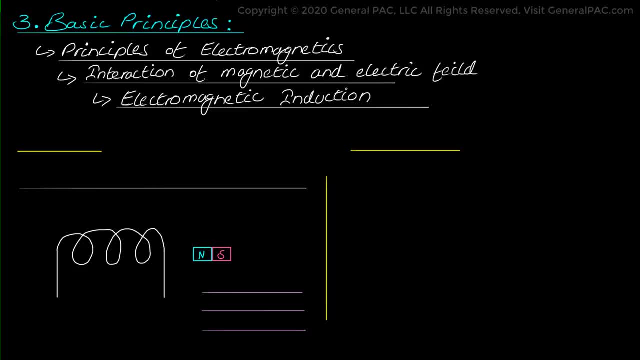 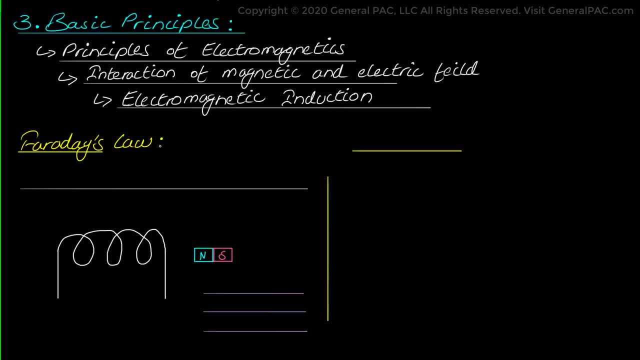 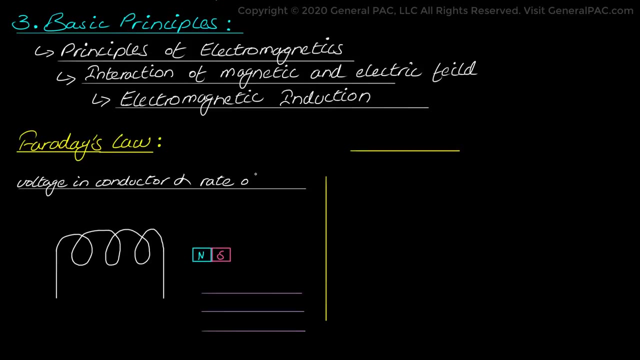 fundamental laws of electromagnetic induction that make machines work, which are Faraday's law and Lenz law. Now, according to Faraday's law, the EMF, or voltage induced in a coil or a conductor is directly proportional to the time rate of change of magnetic flux linking the coil and the negative signs. 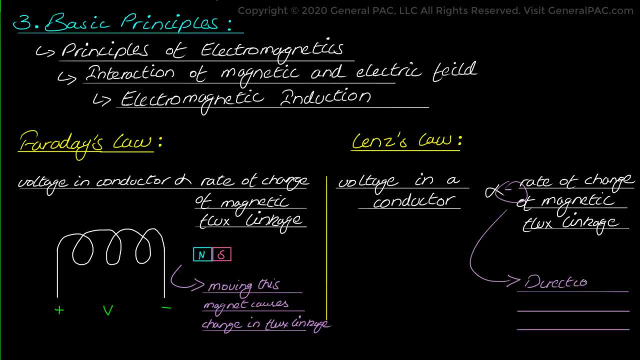 implicated in the magnetic flux are these two. The negative signs are the voltage that Lenz law would suggest that the direction of the induced current is such that it opposes the change in flux producing it. So, as previously discussed, the interaction of magnetic field. 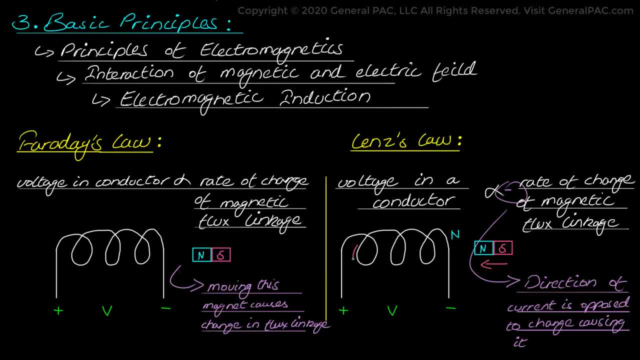 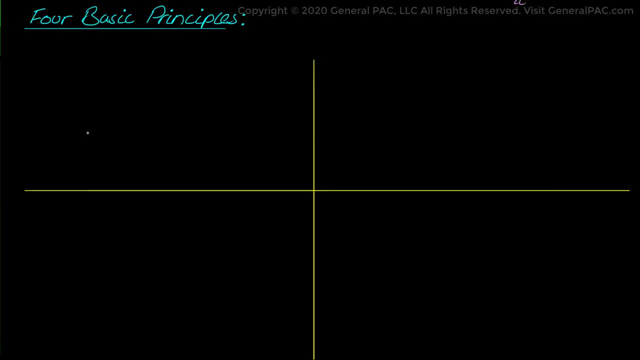 with its surrounding is a basic mechanism by which energy is converted from one form to another form in motors, generators and transformers. Four types of principles describe how magnetic fields are used in these devices. Number one: current carrying wires produce a magnetic field in the area around it. Number two: a time-changing magnetic field induces a voltage. 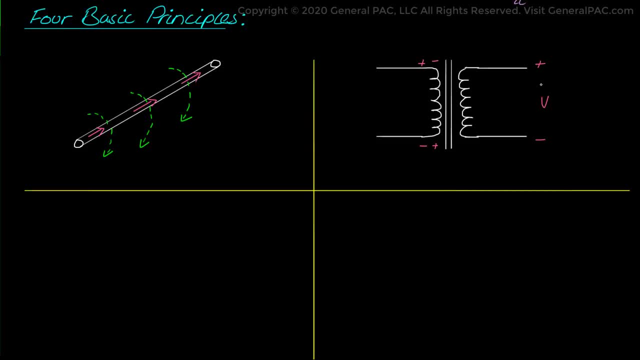 in a coil of wire if it passes through that coil. This is the basis of a transformer action. Number three: a current carrying wire in the presence of a magnetic field has a force. Number four: a moving wire in the presence of a magnetic field has a voltage induced in it. 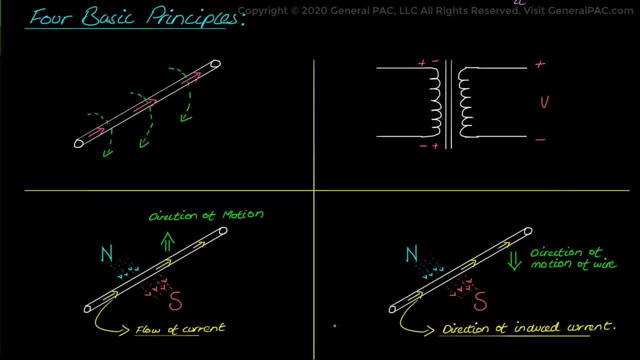 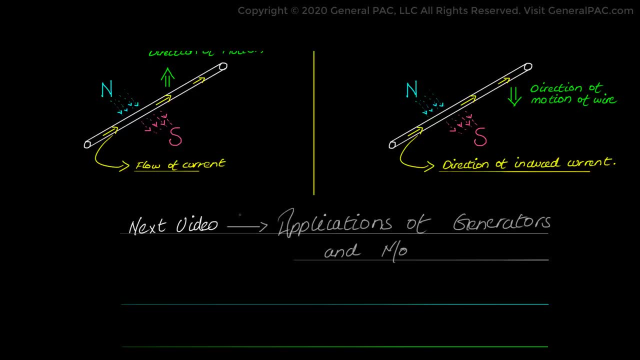 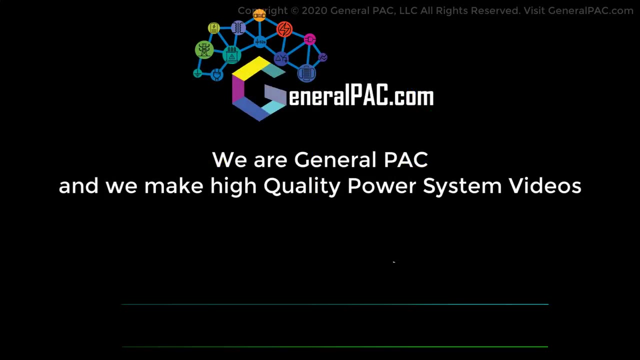